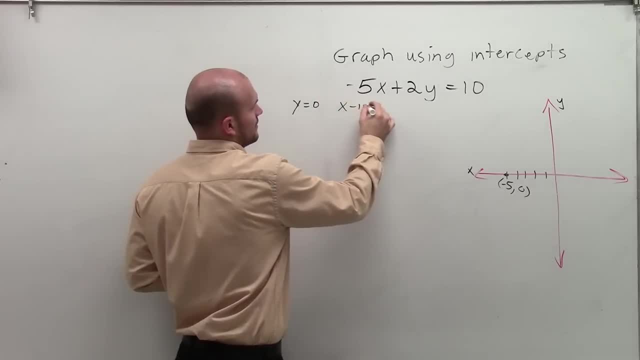 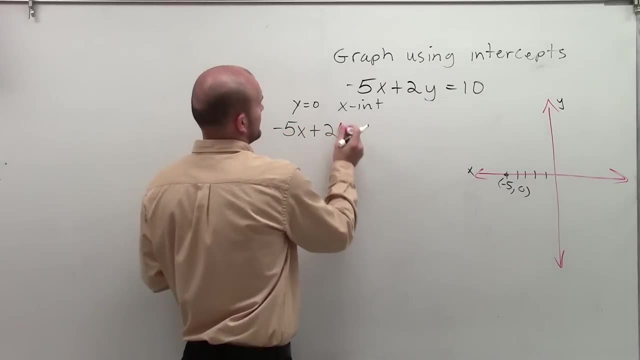 y equals zero. then I'm trying to find my x-intercept. So that's what you're going to do. You're going to do negative. 5x plus 2 times zero equals 10, all right, So 2 times zero is pretty. 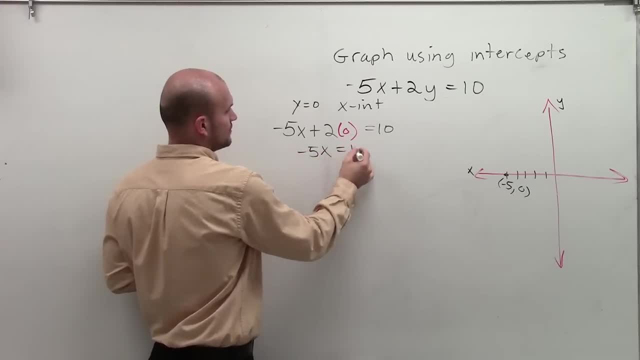 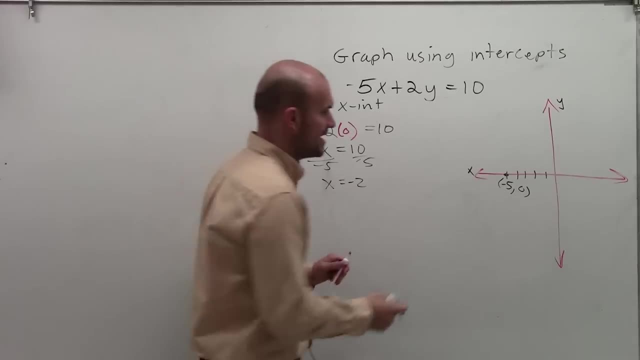 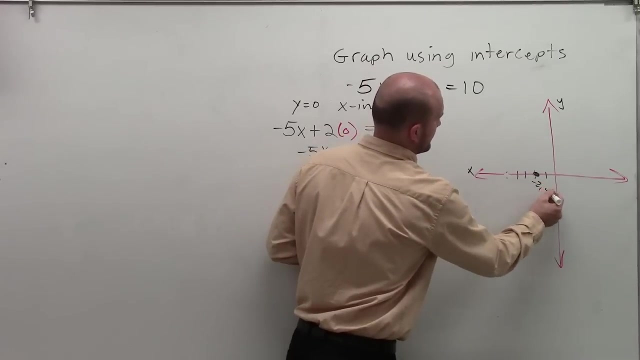 easy: it's zero. So I have negative 5x equals 10, divide by negative 5,, right, And then you have x equals negative 2.. So for actually to graph this- that was just an example- my x-intercept is at negative 2.. A lot of times we like to make sure we just plot it. 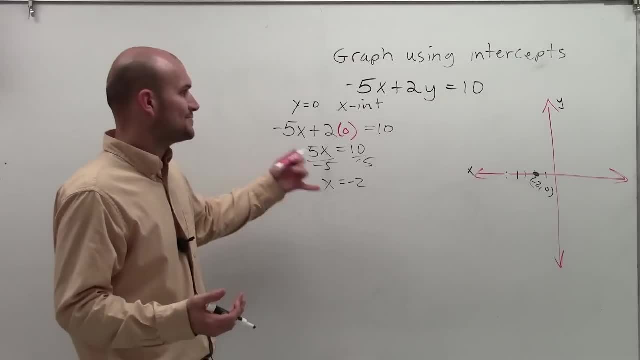 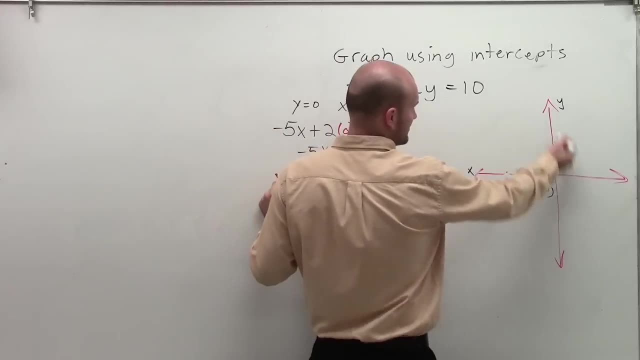 put it in there, right, Cool, all right. So then guess what? So, to find the x-intercept, I put y equals zero. What do you think you're going to want to do for the y-intercept X equals zero? all right, And think about it Right here. what's the x-value on this intercept? 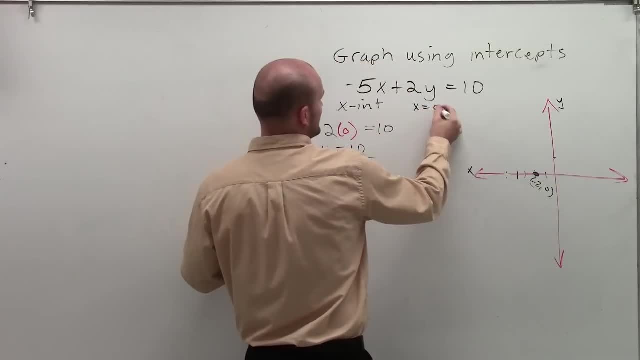 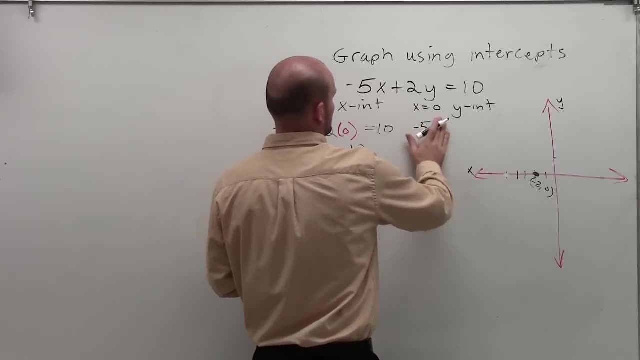 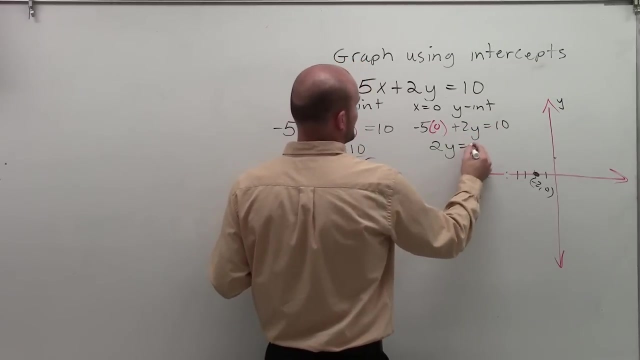 wherever it crosses Zero, right. So we say x equals zero for the y-intercept, all right. So then I just do negative 5.. Times zero plus 2y equals 10.. So therefore I get 2y equals 10, divide by 2, y equals 5, right. 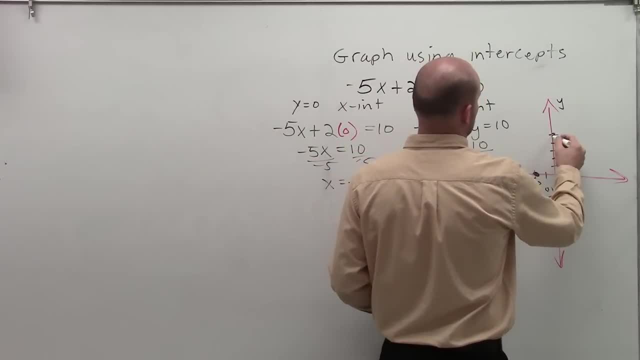 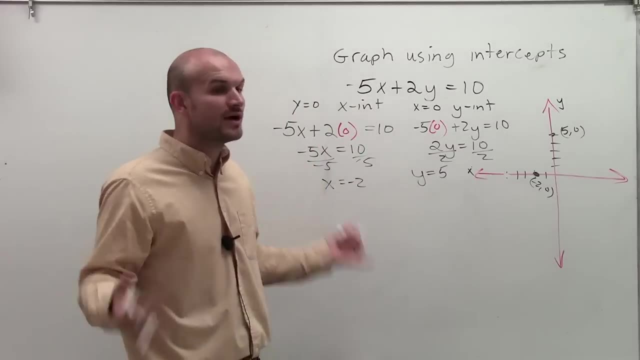 So then I go up 1,, 2,, 3,, 4,, 5,, 5,, 0.. So, now that I know that I have an x and y-intercept, remember to graph a line. all you need is two points, right? So just connect. 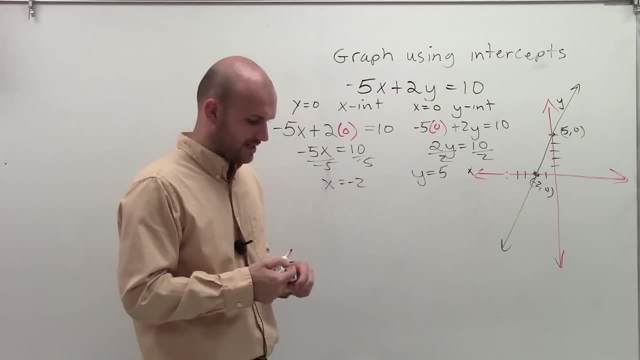 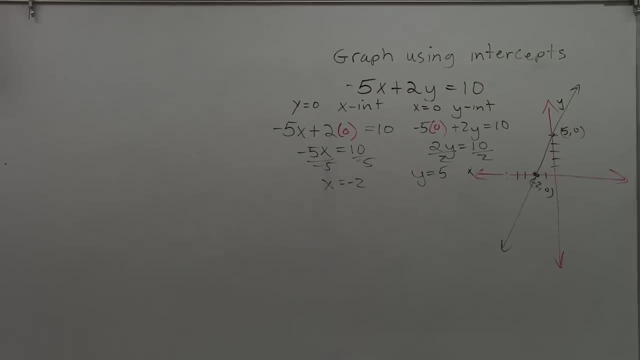 And there you go. That's it. That's all you got to do. So that's how you graph using the intercepts. So that's the fun way.